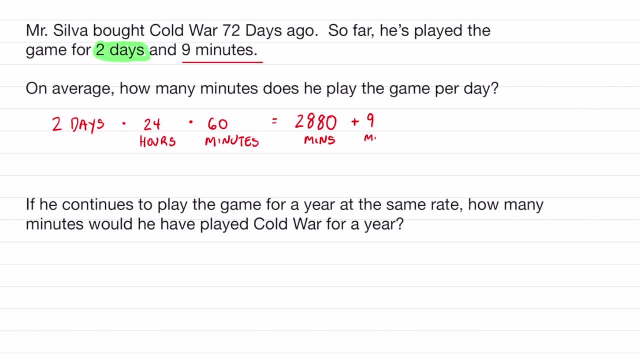 So I have to add nine more minutes and I will get 2,889 minutes. However, I played that game for 72 days, So really easy step. All I got to do next is divide that by 72, because I played the game for 72 days- and I will get about 40 minutes- 0.125.. 40 minutes a day. 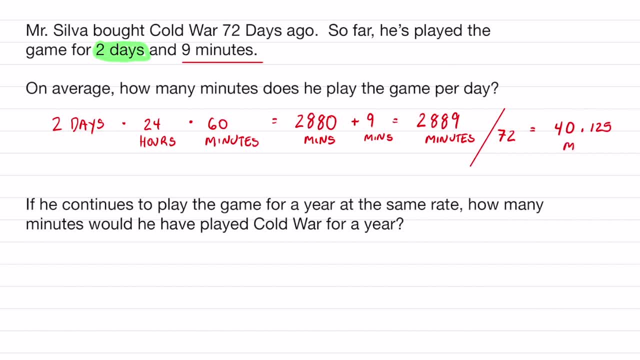 that I played that game for 72 days. That is crazy to me. That is actually the first time I calculated that. Let's say, I continue to play this game for a year At the same rate. So this is a great ratio question. How many minutes would he have played Cold War for a year? 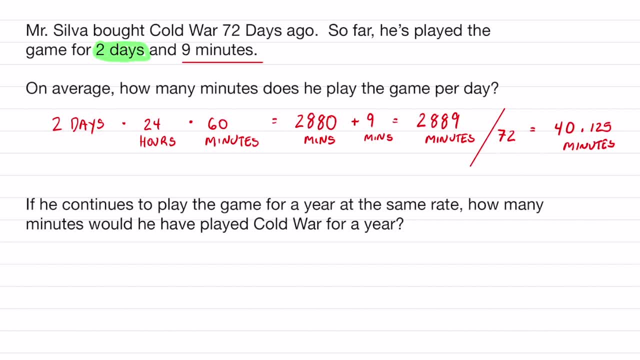 And I'm actually really nervous to find this out. So let's take a comparison here. Let's take 2,889. That's the minutes that I played the game over the number of days I played it. If I kept going at this rate for a whole year, which is 365 days, that is what I'm going to put at. the bottom. Then I can figure out how many minutes I'm projected to play this game for an entire year. All I have to do at this point is your favorite thing to do: Cross, multiply and solve for X, and I will get my projected minutes for the entire year. Let's do that: 72 times X is 72X, 2,889 times 365.. That equals. 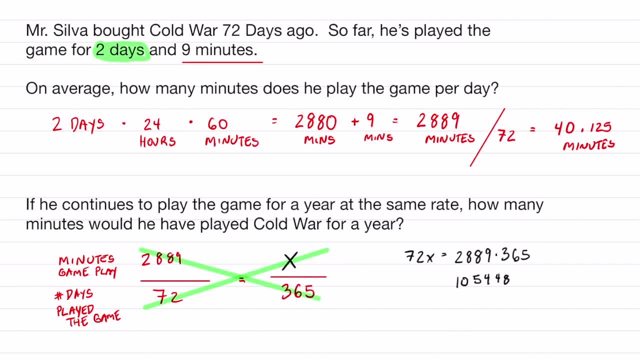 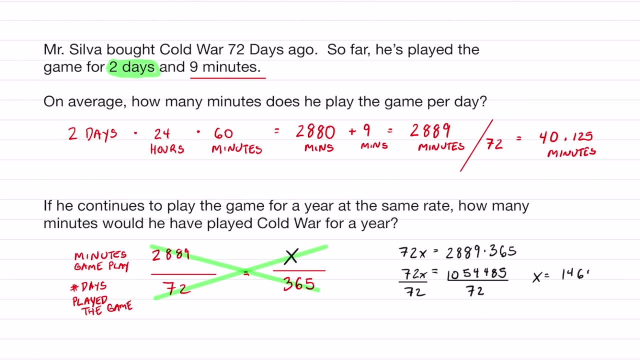 1,054,000.. 485.. And then the last step is just to divide both sides by 72. And I will get the total amount of minutes I'm projected to play this game for the entire year If I continue that same pattern: 14,645 minutes- 0.625.. 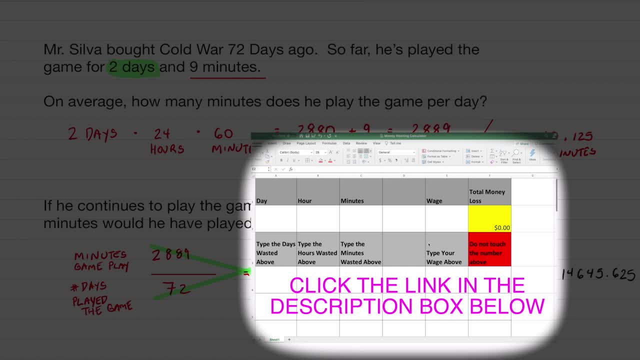 Let me show you how my money wasting calculator works. You can access this for free and calculate stuff for fun. But let's say I type in my projection expected yearly minutes that I would have played Call of Duty 14,645 and 625 minutes. You're going to type that there And this box for wage you can actually put whatever wage you want to put. 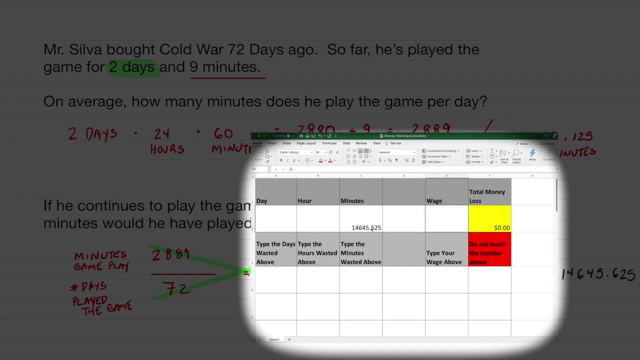 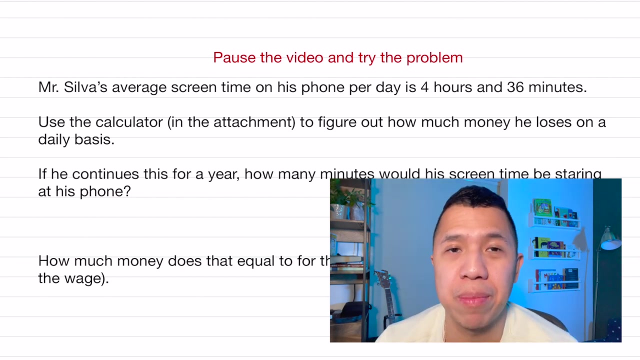 Let's just pretend we're doing $15 for minimum wage. That equates to $3,661.41.. Wow, I'm really embarrassed to share this statistics. but let's go back to the beginning. Let's go through my phone and see my phone time on a daily basis. 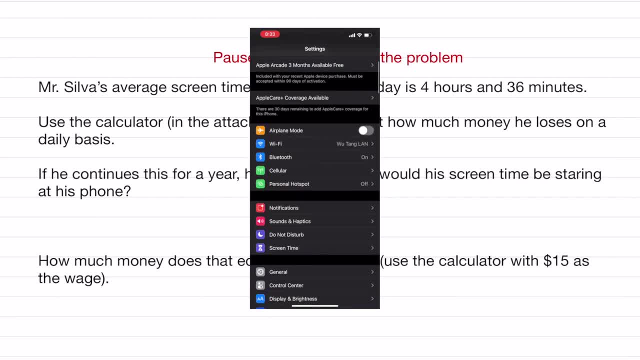 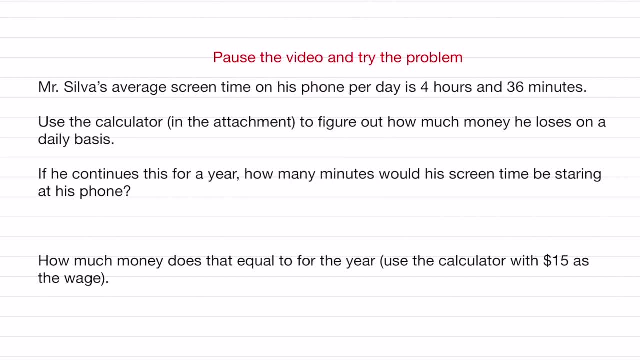 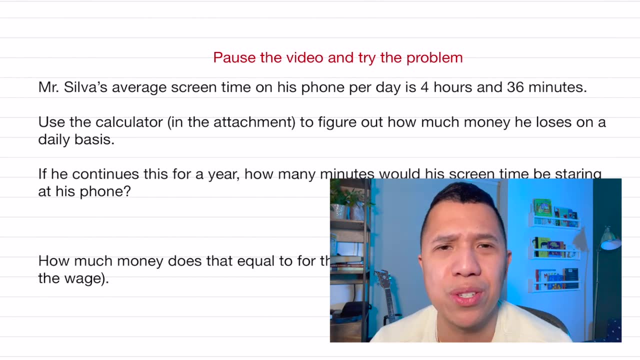 If you got an iPhone, all you got to do is hit settings, find where it says screen time, click that. But mine is 4 hours and 34 minutes on a daily average. Pause the video and try out this problem. When you're done, just unpause it and see how much money I wasted if I were to continue my phone screen time for a year. 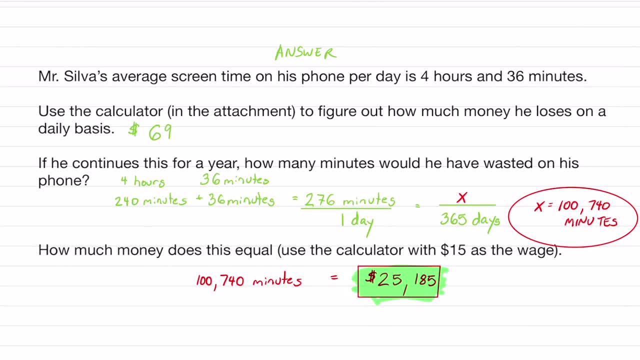 Don't cheat. Remember that you can access that calculator in the description box, And that is about $69 a day, To be honest. you could just multiply this number by 365 to get this number right here. But what would be the fun of that? 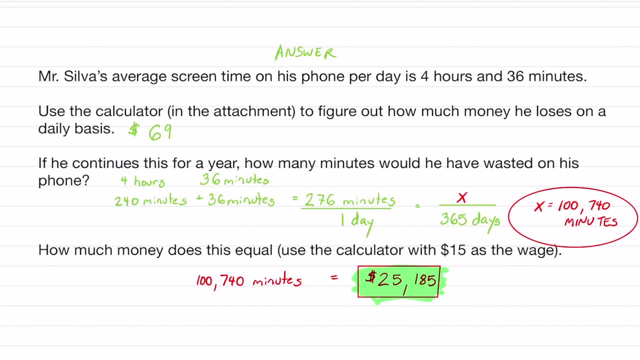 I want you guys to learn about ratios. The second question is: if I continue this pattern, how many minutes would I have wasted on my phone? I mean, it's not a full waste, you know, because I make these videos. but no excuses. 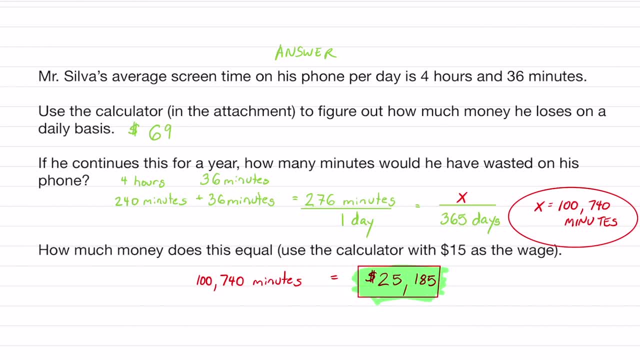 Sometimes I do waste a lot of time on my phone. 4 hours and 36 minutes. First you have to convert this into minutes And all you have to do is times that by 60. And then add these two up and you'll get the minute amount per day. 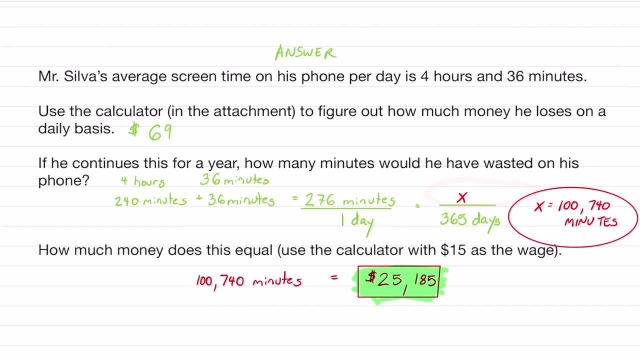 The projected minutes that I'm going to spend on my phone. all I have to do is set up a proportion like this: Cross, multiply and solve for x, And I will get 100,740 minutes If I use my calculator. This is mind blowing. 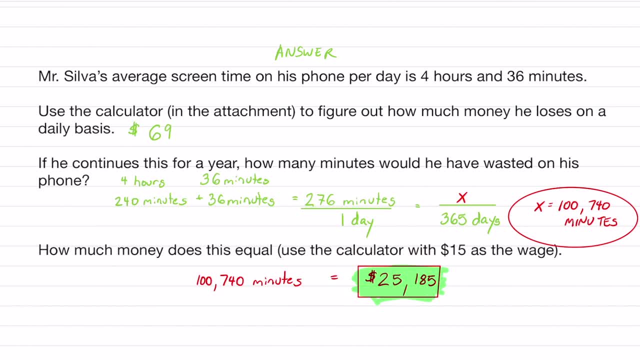 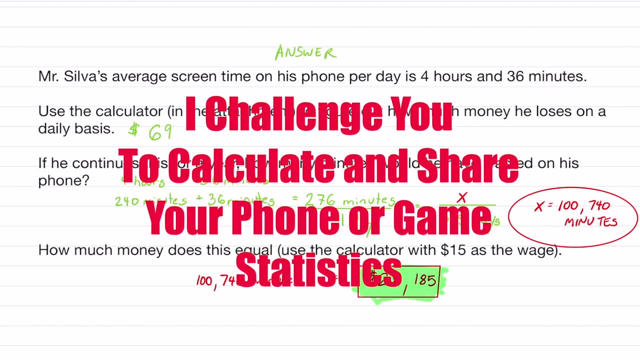 That's about 25,185. if that's me making $15 an hour, which is about to be the minimum wage, I dare you guys to put in the comment box what your amount of money times $15 an hour will equal if you calculate your phone time for a year. 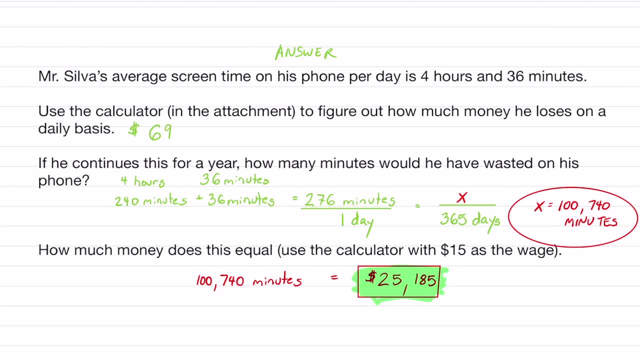 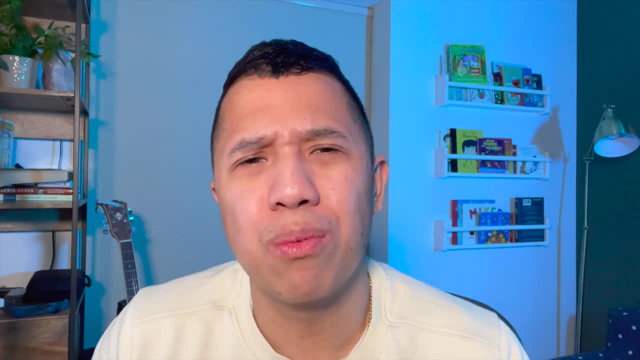 I dare you, I will pin the highest score, and I think that'd be pretty funny. Watching this video really made me think about how much time I've lost spending with my family And watching my kids grow up. They grow up so fast. 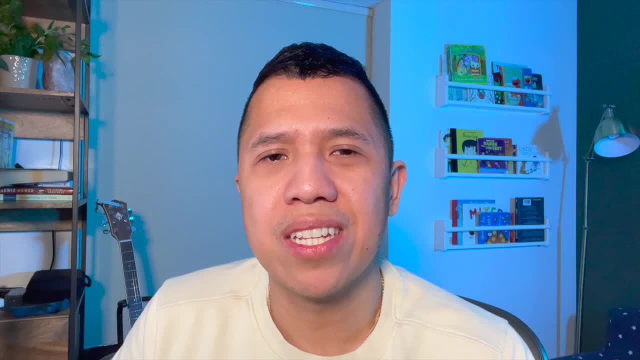 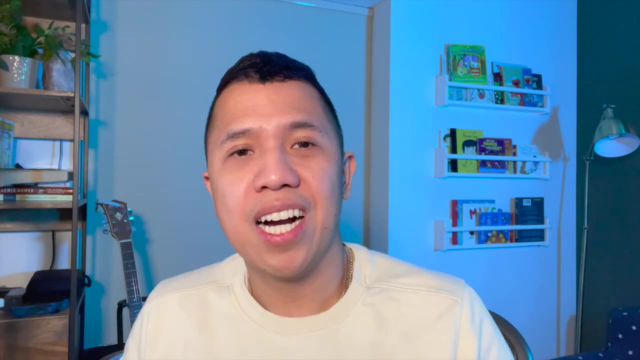 And I hope you really enjoyed this video. Anyways, if you did make sure you throw me a thumbs up And if you have any ideas for other videos, let me know in the chat box below. I hope to see you guys on the next episode. Peace. If you're an organization or an individual that need to manage many real estate properties, then this application will be ideal for you. Hi guys, my name is Akshay and welcome to AppDNA, where we talk about all things: apps. The application that we are going to take a look at today is Property Manager, and we'll be using Zoho.